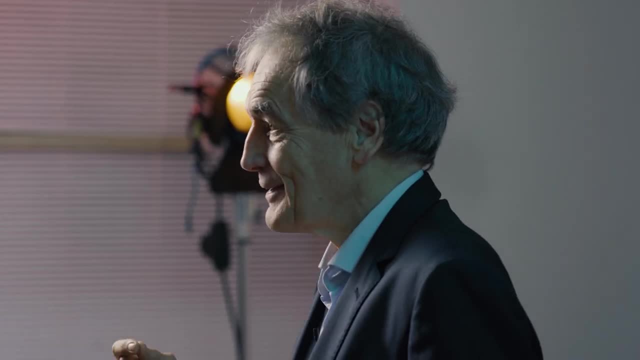 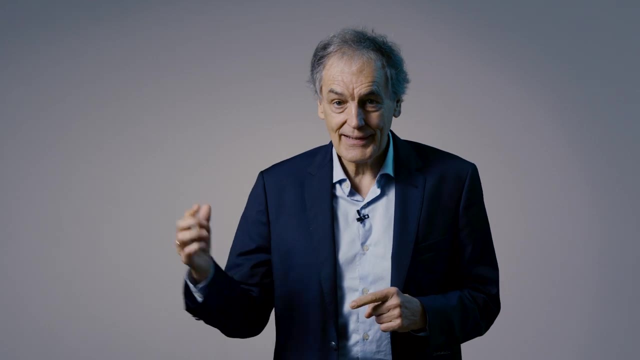 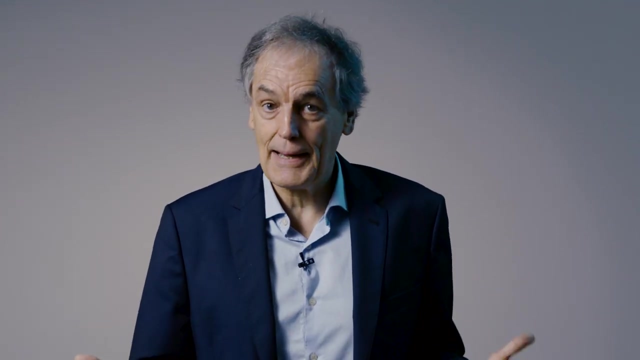 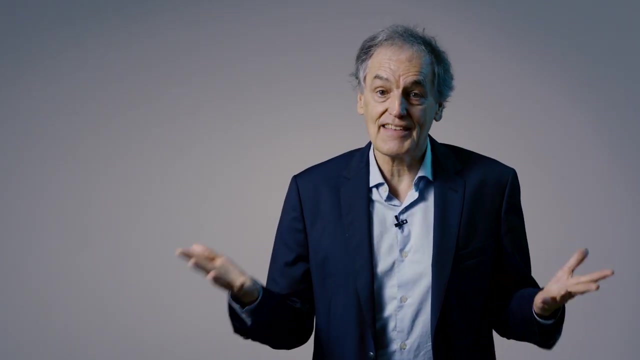 This is obvious, But somehow a computer is a thankful object. Thanks to computer science and thanks to those powerful machines, a new era started in mathematics, New disciplines of mathematics made possible by the development of computer science, And one of the most famous examples of this is what we call the fractal geometry. 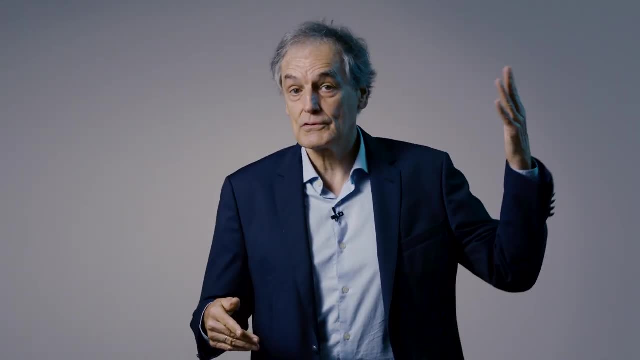 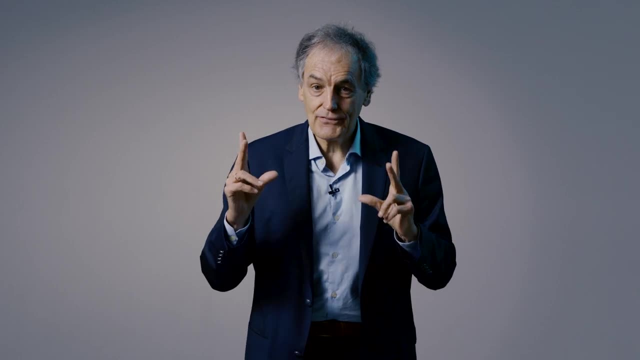 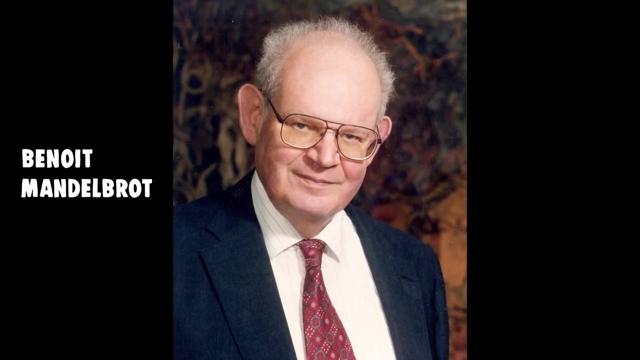 Geometry was developed a long, long time ago. We have talked about Plato and Pythagoras and others, And thanks to the computer, a new kind of geometry became possible, And the founder is Benoit Mandelbrot, a French genius. 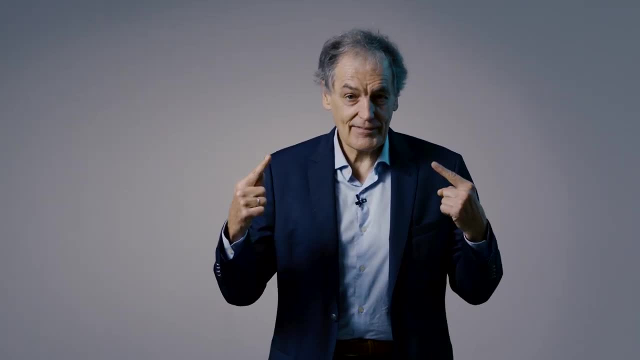 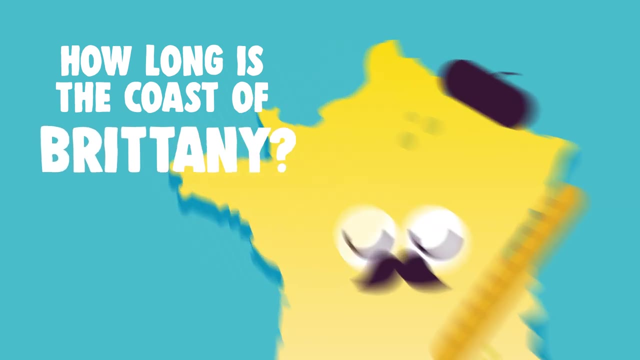 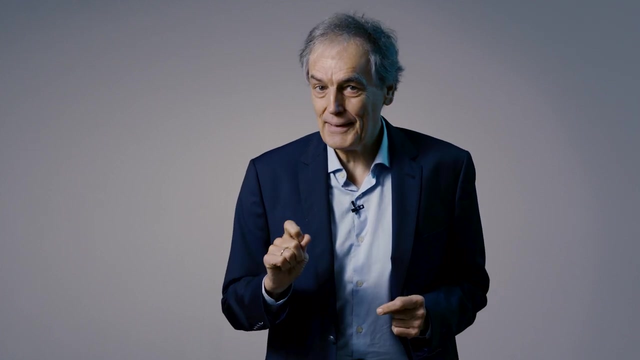 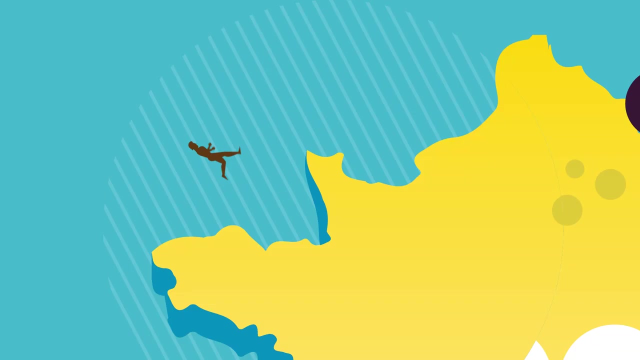 worked as an IBM fellow And he started his research with a very peculiar question: How long is the coast of Brittany Looks obvious. Where is the problem? But the answer of Mandelbrot was unexpected. The length depends on who you are. If a human being, you walk the coast of Brittany. 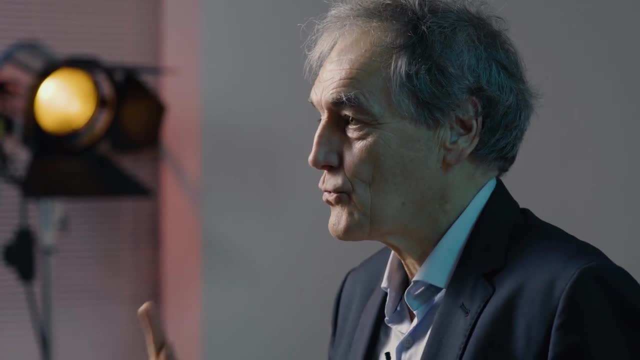 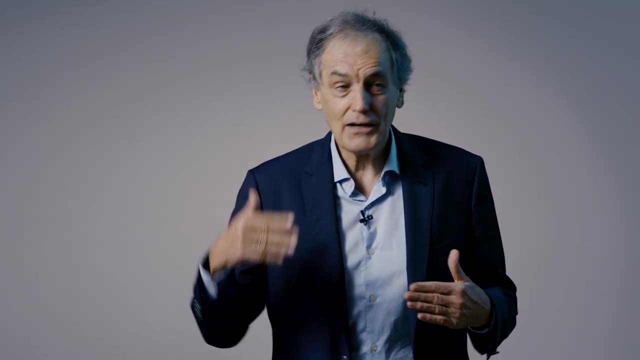 and you have how many kilometers I don't know. But if you're a rabbit, for example, and you follow the path, the coast of Brittany is going to be a longer path. Now imagine you are an ant. You have to do like this. 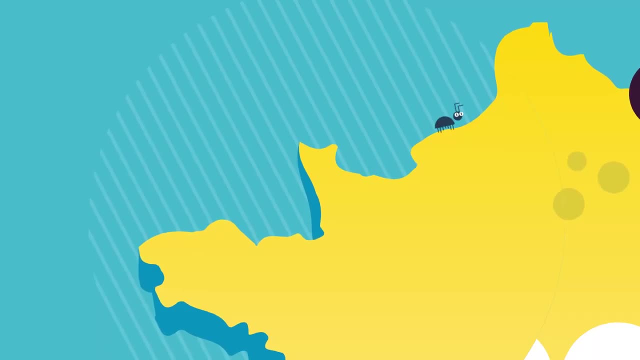 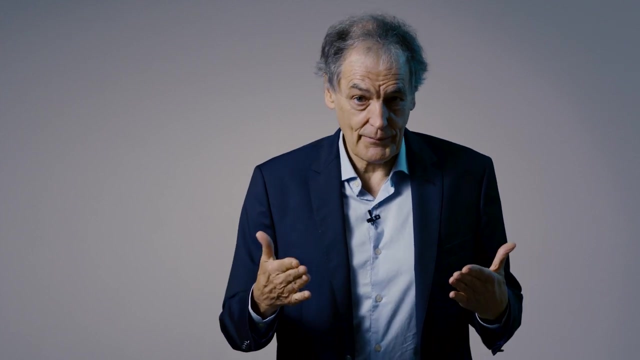 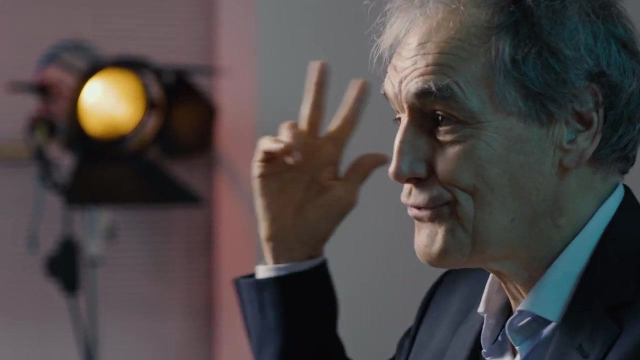 To just follow the coast of Brittany, And that was a starting point of Mandelbrot. Another thing is, if you look at this coast of Brittany, what the ant can see is similar to imagine an astronaut from outer space looking at the coast. 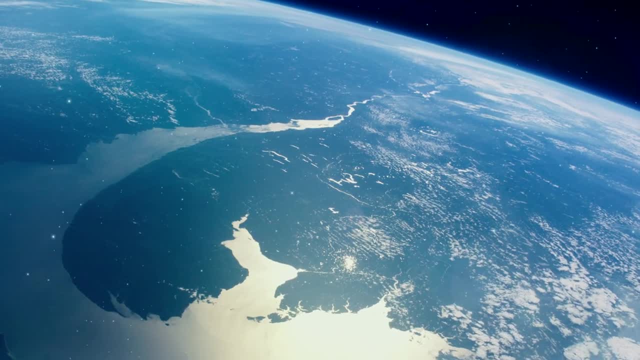 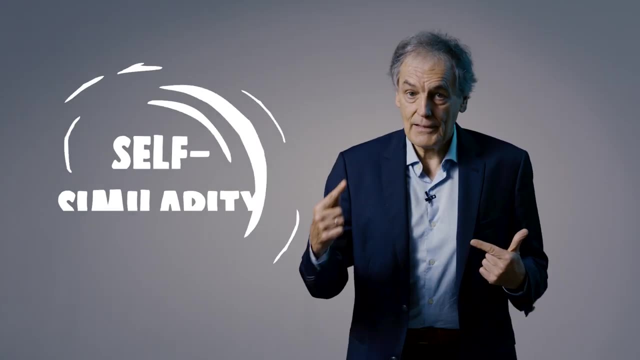 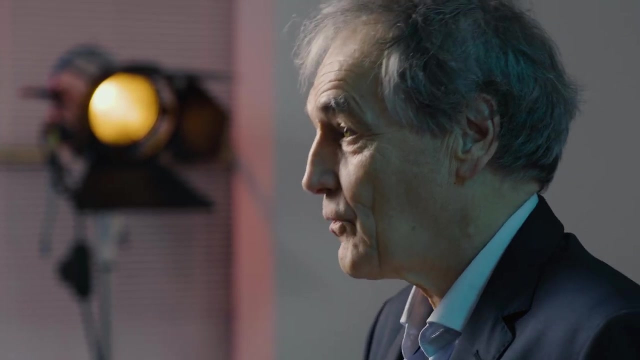 The ant and the astronaut see the same thing. The only difference is the scale, And this is called self-similarities. Self-similarity is a property of an object which looks the same whatever the scale, And that's how Mandelbrot starts this new geometry. There are many famous examples. Let's 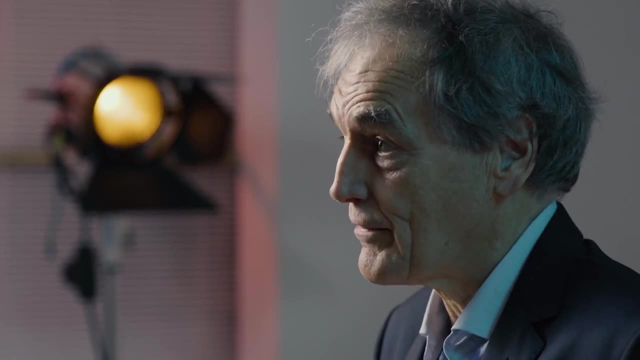 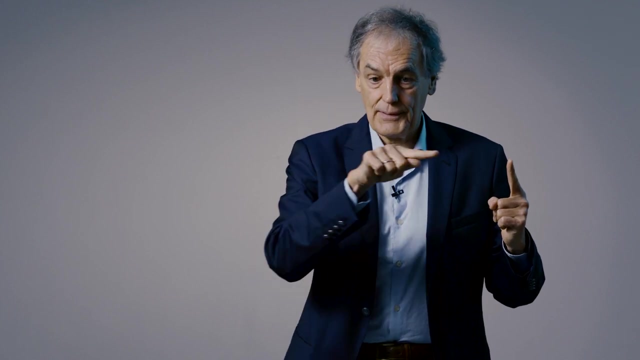 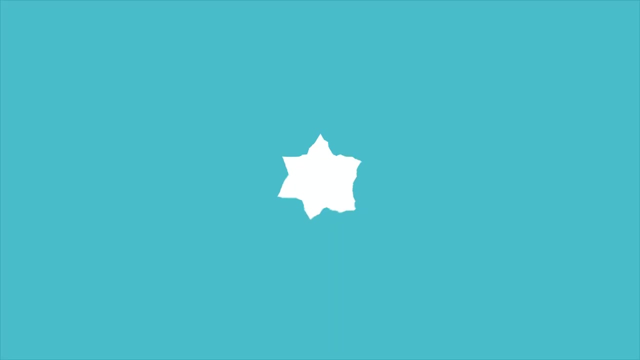 take two of them. The first is the snowflake. If you start with a line like this, a segment of line, And then you do this, You just beat like a triangle And on the side of the triangle you beat the triangle And then you beat it. You always build a new triangle in the middle of the side.